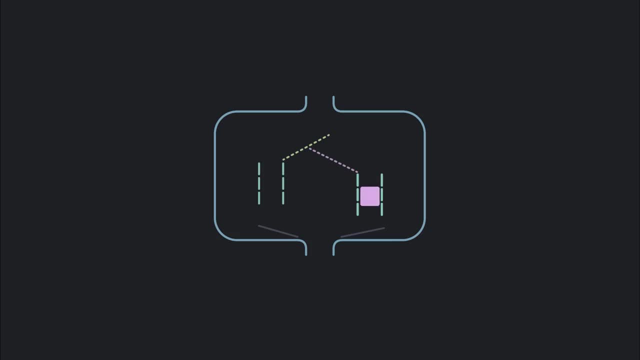 No thing inside of the function that isn't directly derived by the input. Once you introduce state, the outcome of the function can vary based upon that state. Honestly, most programming paradigms are really just different takes on how you manage state. It's all about state. 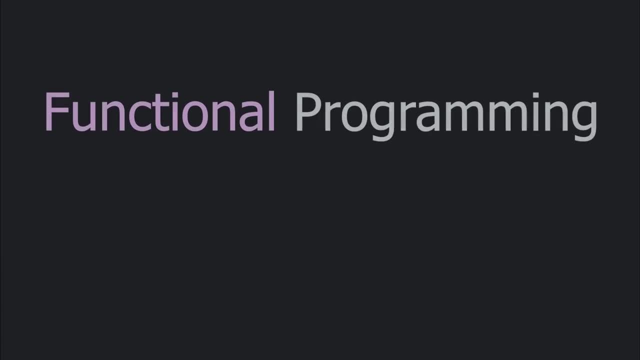 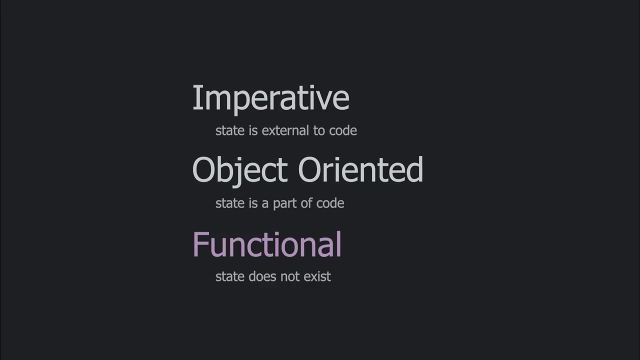 So let's talk about what functional programming is, why it kind of sucks, but why adding a little bit to your code is awesome. Functional programming takes one extreme side of the state opinion. It's about writing programs based upon one core concept, concept. There shall be no state. You have inputs which are transformed into outputs. 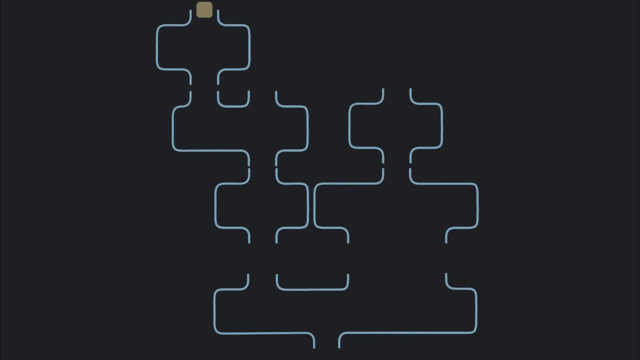 In order to get stuff done, you compose and connect functions to other functions, hooking up their inputs and outputs together into one big, long chain that achieves the goal of the program. But you don't have objects or structures in memory that you mutate to. 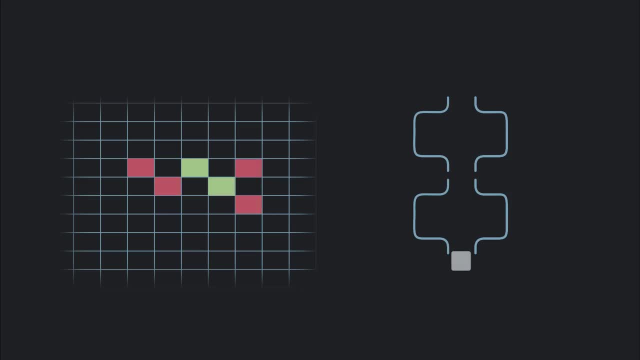 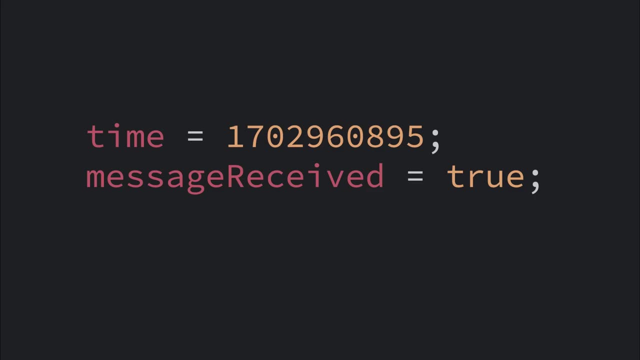 track what's going on In this absolute, pure world where you want to write functions with no state. this also means that you're not allowed to mutate variables, So this means if you were to set a value, you cannot change it again. This means conventional iteration. 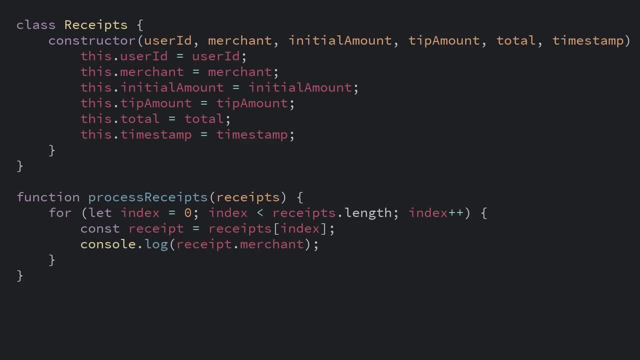 loops like for and while are impossible. If you think about a for loop or while loop, it requires you to mutate some state, at least some variable that's tracking how many times you've iterated. So how do you do a loop in a pure functional way? The answer: with functional. 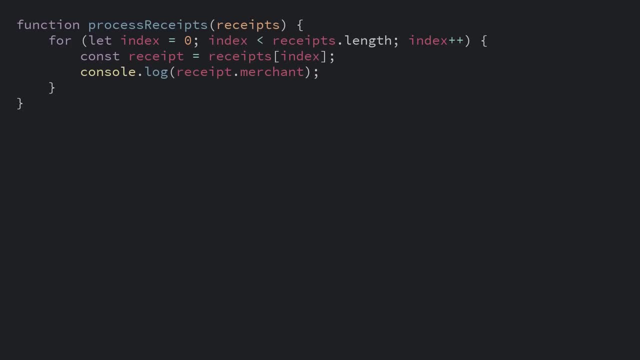 programming is usually well more functions when all you have is a hammer. This is the part that we want to repeat over and over again, So we'll just pull that part out to a function. So now we need to replicate the three parts of the for loop. The key thing that the for. 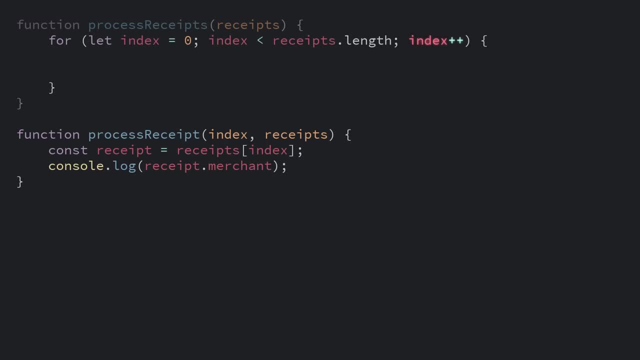 loop does is increment the index variable so that the body gets rerun with each index. So we need an equivalent of incrementing index and rerunning our body inside a process receipt. Since we can't mutate index, you can imagine us creating a new variable, next index. So 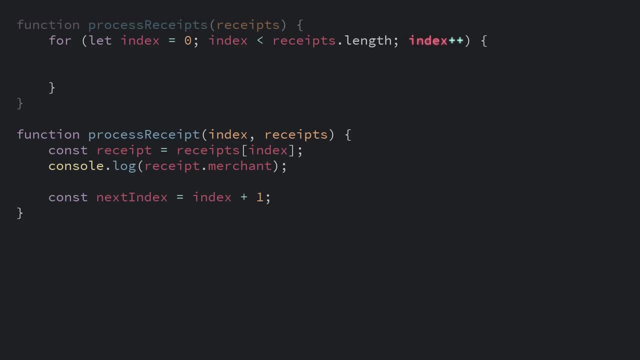 we'll call it processReceipt, which contains the next index we want to process. But now we want to repeat this section again, So we'll need to call processReceipt again. So now, if you were to call processReceipt, let's say, with an index of two, it would print the. 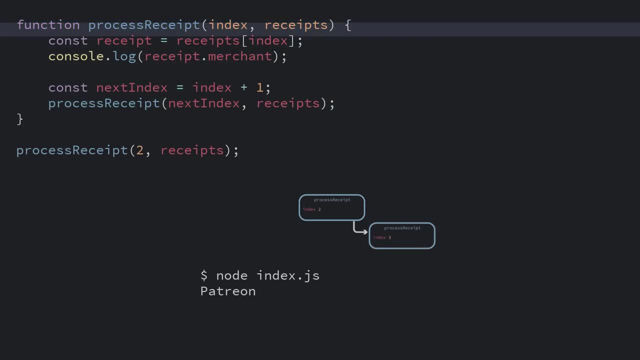 merchant from index two, then recall process receipt with index three, then four, etc. But as it is now, it'll keep calling the process receipt forever until it goes beyond the size of the array, causing an error to be thrown. And this is where the second part of the for loop comes into play. the condition We only 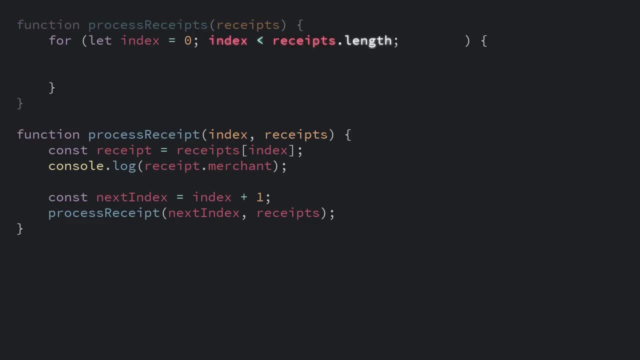 want to execute the body if the condition is met. Otherwise we do nothing and move on. So we'll move that condition down into our function, where we only do anything if our index is still in range. You can see when we run the program. it works like before It. 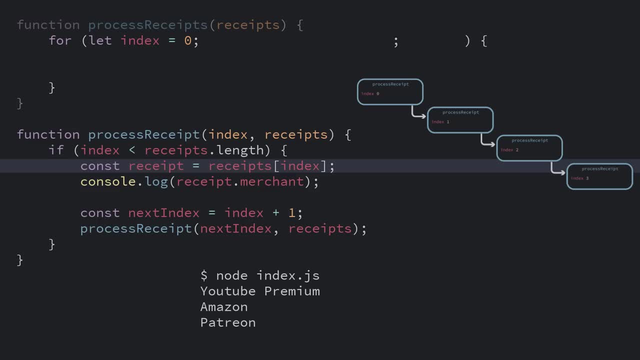 increases the index beyond the size of the array and we still call our function. But in this case it fails our condition and we do nothing. This breaks the recursive loop and all our functions return. Recursion is just a fancier form of iteration. 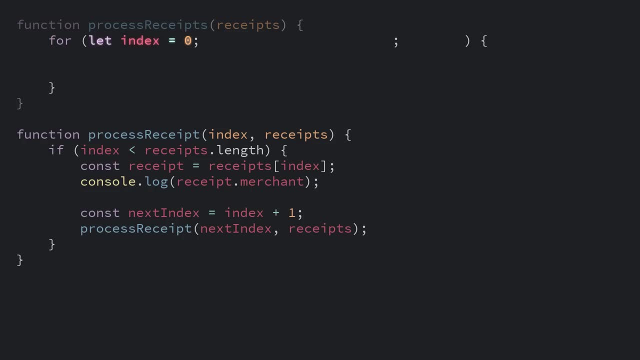 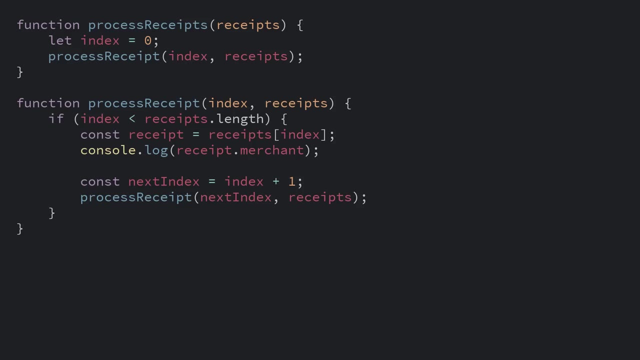 And finally we have our last part of the for loop, which is where we set our starting point. This just represents our first call into our recursive loop. So now we've completely converted our loop to be done in the more functional way. We can also remove any unneeded variables. 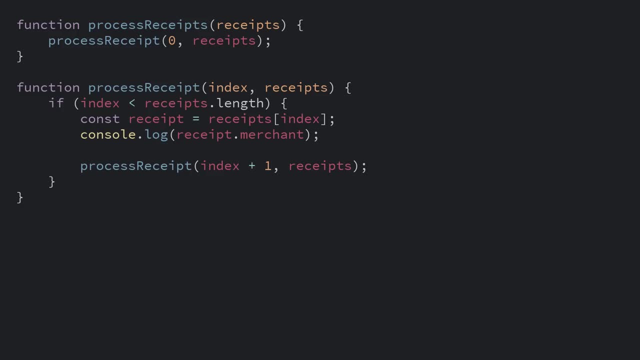 to make our code more concise, if we wanted. OK, OK, this is pretty simple and just logs each item in the loop. But what if we wanted to do something useful, like finding all the receipts that belong to a particular user and return them so they can be displayed elsewhere? Well, we can take the user ID as a third parameter. 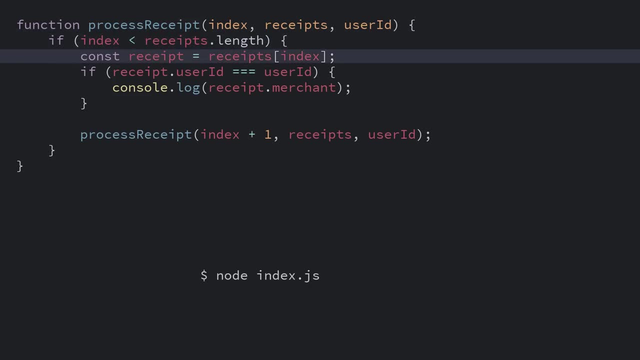 and then check if the user matches. This now only prints the receipt of the merchant if the user ID matches, But instead we want this function to return the list of matching receipts so that it can be displayed on the web app. We need to somehow return the 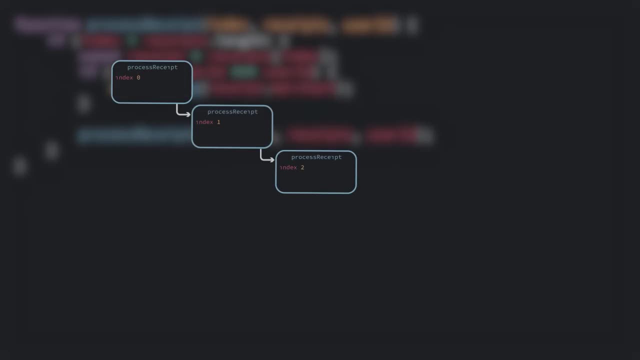 results of the matching At each recursive call. we want to make an array with the current receipt at the front and the results from the deeper calls attached at the end. This way we can get back everything in order. But we only want to append the current item if it has the right user ID. Otherwise we just want. 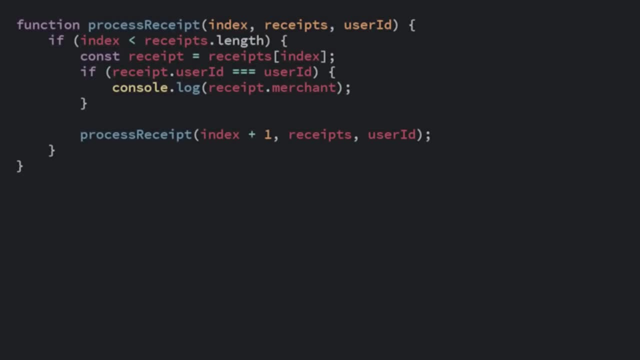 to pass through the previous result. So, in order to do this, we'll actually get the results of the deeper calls first And then, if the user ID matches, we'll return the results to the same line and we can do the rest in the future. 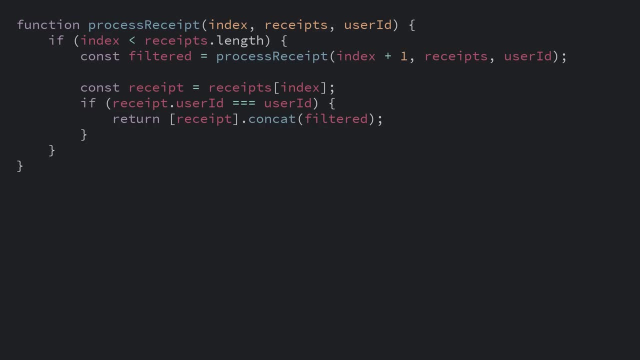 OK, so we're done with the recursive calls. Now we can examine our recursive call process, the current results appended to the later results. Otherwise, just forward on the later results as is. And lastly, if we've processed the entire list, we'll. 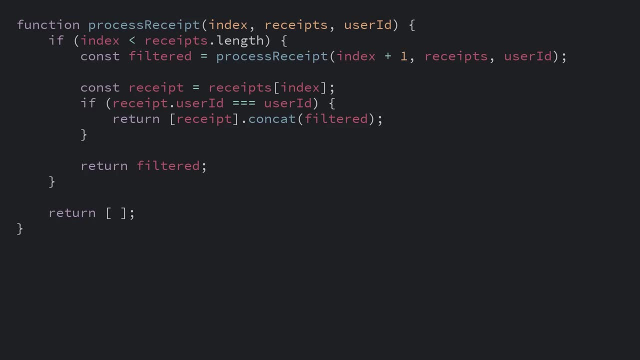 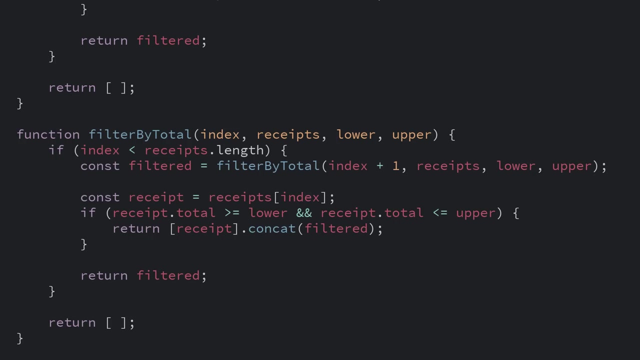 just return empty results, since there's no more results to be had. So now this function just returns all the receipts for a given user ID, and we'll give it a better name. Thing is, you could imagine this pattern happening over and over again whenever you wanted to find stuff in an array. The only difference between 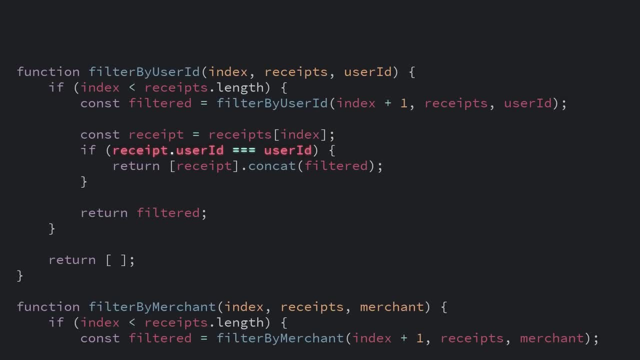 these functions is the condition in the if statement. We could replace all three functions with just one. if we instead passed in a function that returned whether or not an item should be included. Let's pull out the condition and move it to its own function, And instead of taking the user ID as a 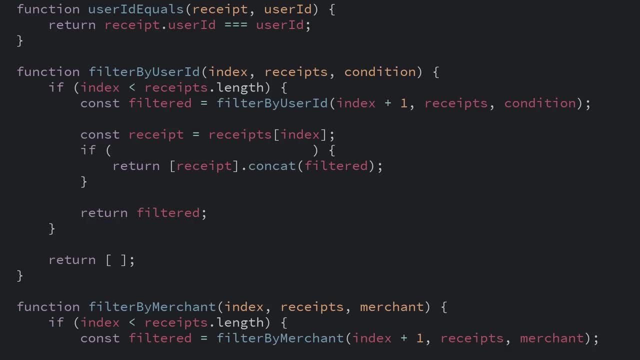 parameter. we'll pass in that function. instead We can call it condition or, if you want to be a classy fellow, you can call it predicate. Then we just call that function where the condition used to be, and that's it. That function tells us whether or not to include the item. Then we can pass our 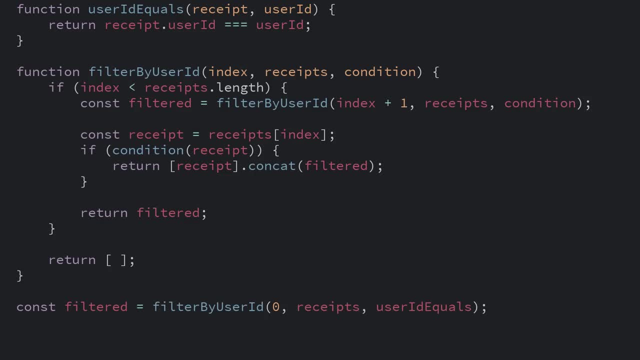 condition the user ID equals function into our filter and of course we can now rename our function to be a generic filter. Now we can run our beautiful program with our filter and user ID equals function and wait, we have a problem. Our user ID equals function takes two parameters: the receipt and the. 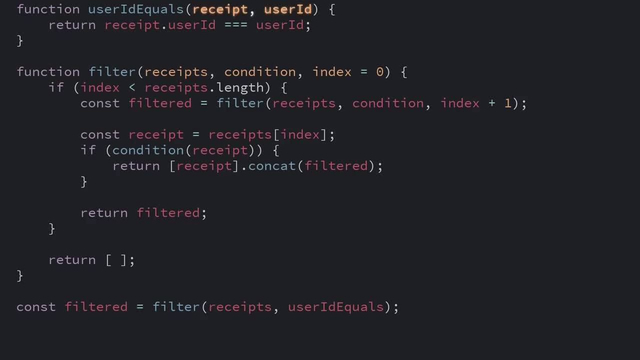 user ID to check against, But our filter function only checks against the receipt itself. We don't know the user ID to check against. We could try passing in another value that we could relay into the function, But what if we need more than one, Like in the case? we need to check if the total was between a. 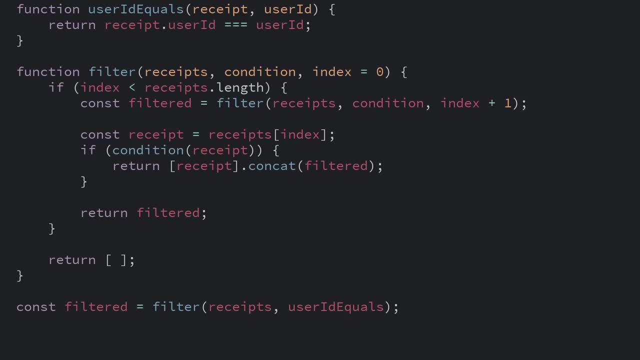 range, It gets a bit awkward. So instead we're going to get a bit fancy here. Instead of having our user ID equals function. take both a receipt and a user ID. We're going to have it. take only the user ID that we want to compare against. 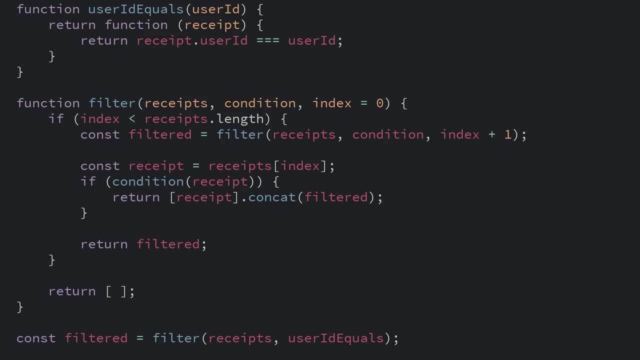 And it will construct and readjust. So we're going to construct and return a new function that takes a receipt and returns whether it's from the user ID. We then pass in that new function that's been created into our filter. This is a little weird, but what's happening is. 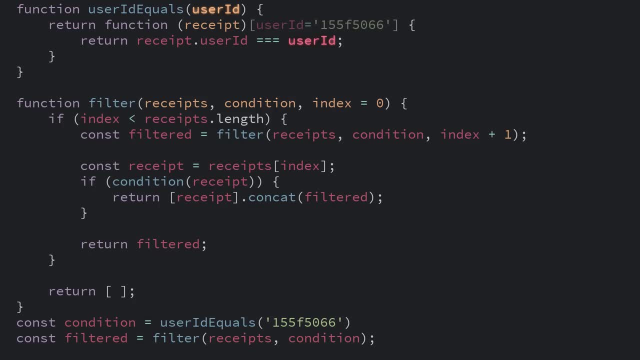 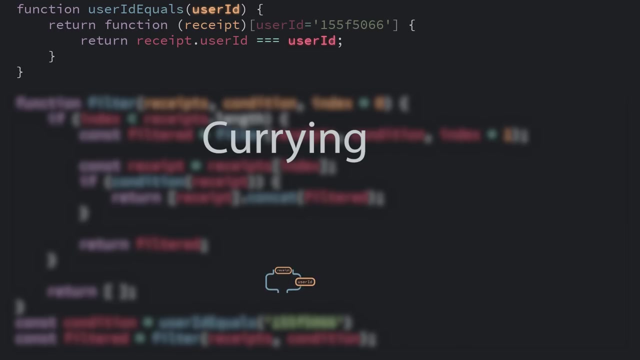 that the user ID is like a secret extra parameter which is bound to the function, And this function remembers that value and can use it. The name for this pattern is called currying. Instead of handling the entire operation at once, it returns a function that handles the next part of the operation. The later part has the 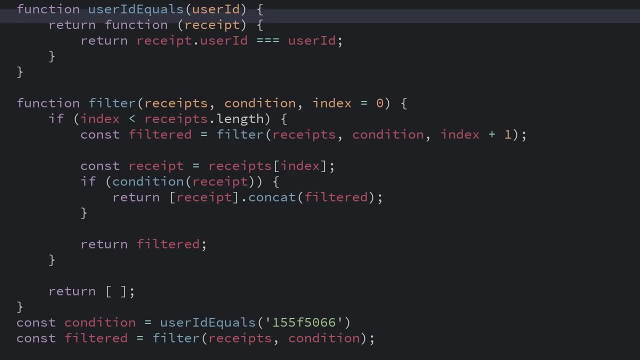 previous state bound to it. That new on-the-fly created function is what gets called when filter needs to check a condition. This is what's a bit funny to me, Because functional programming is supposed to be so different than object oriented programming, But by binding 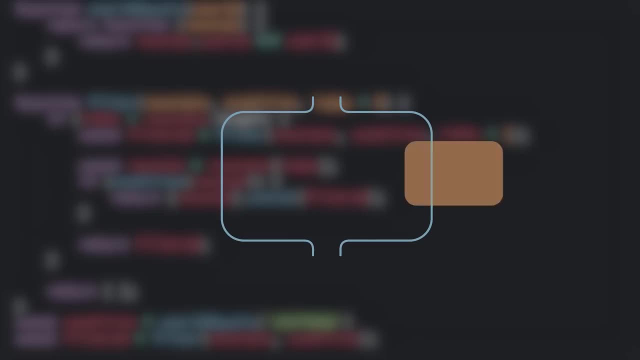 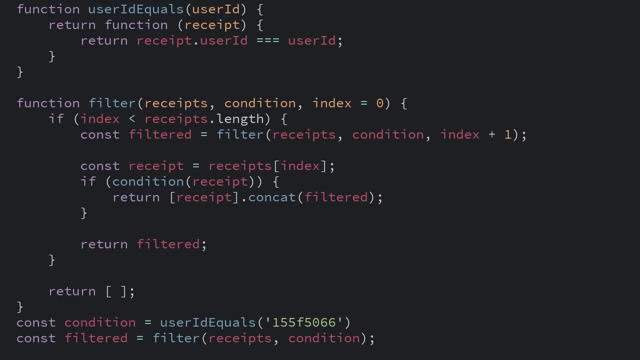 data like this. we're creating an instance of a function with some bound data to work with, Instead of creating an instance of a data object with its bound functions. Currying like this is a bit of an older way of doing this. You can automate this in JavaScript. 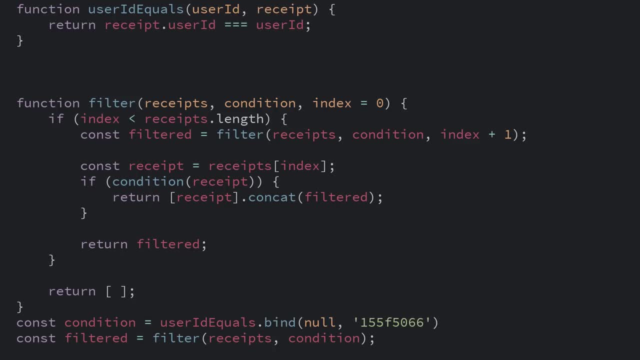 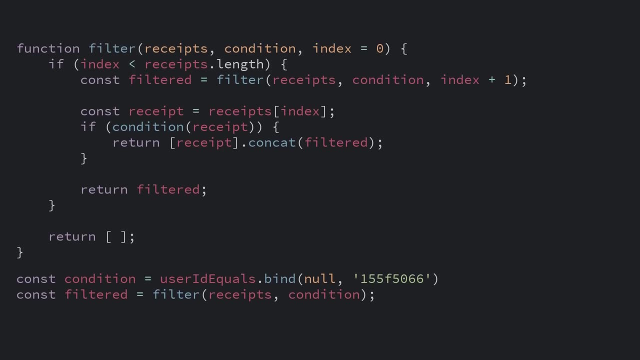 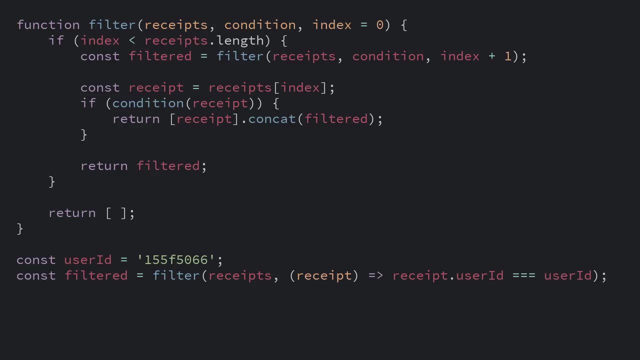 in many other languages by using bind. I won't go into bind fully here, because really the way we want to do this today is to use lambda functions. This is where we'll move our equals check Now. this is finally where things start to get kinda nice. I'm filtering by user now. 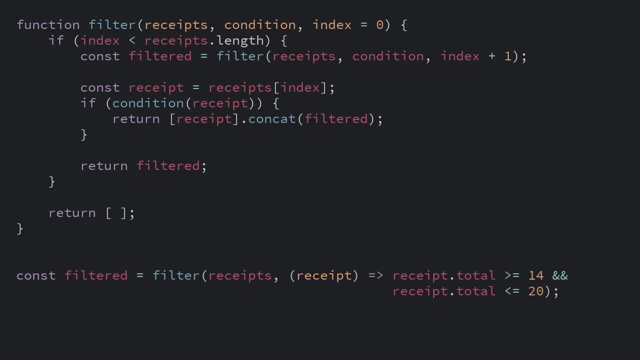 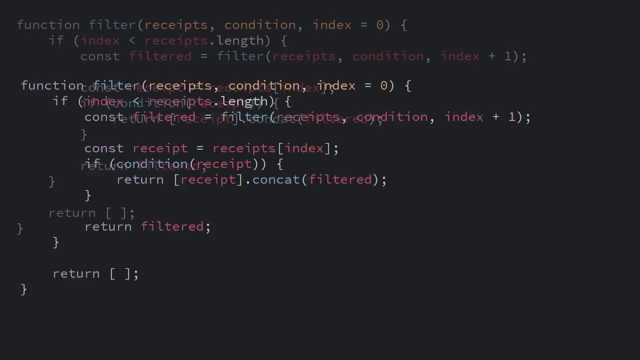 Or I can filter by merchant, just like this, Or do a more complex check on the total. here We might want to get just the filtered merchant names instead of the entire object If we devise a new function based upon our loop that doesn't filter based upon a condition. 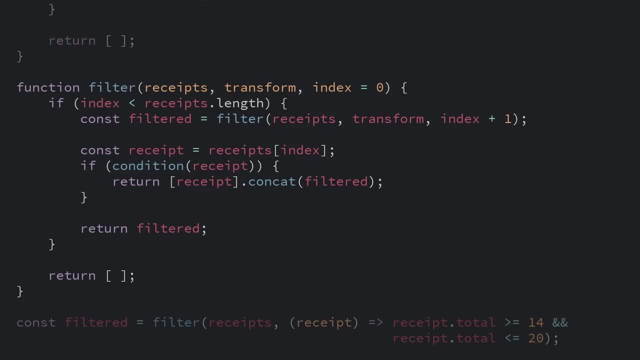 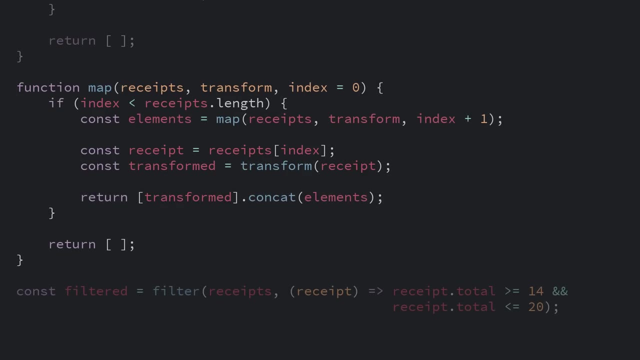 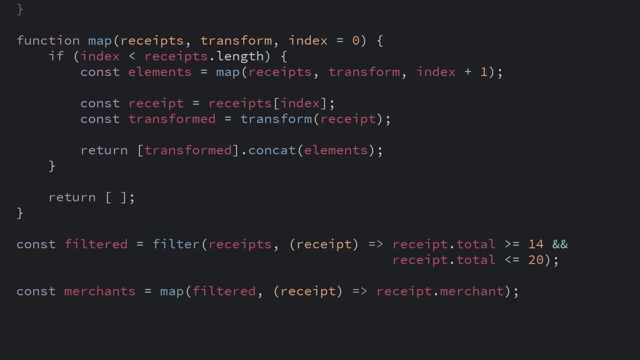 but instead takes a function that gives you the desired result for each element. We insert that new transformed element into the array. instead We'll call this function map, Because it maps each element to a different thing. Then we can chain these together. So first we get our list of receipts, Find the ones. 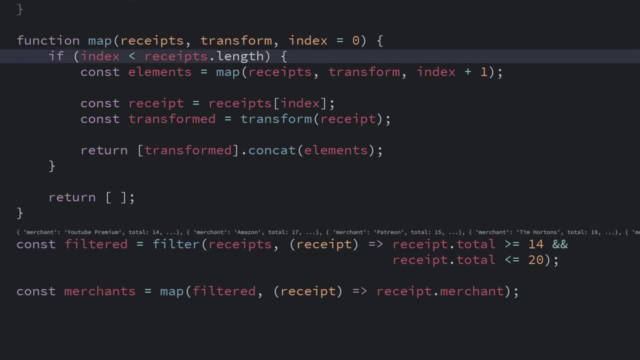 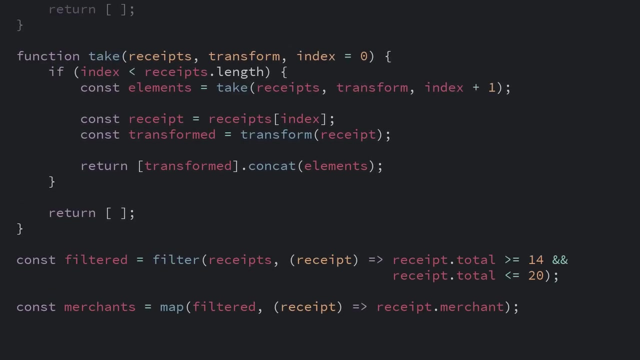 with a total between 14 and 20.. And then just say: for each, give us the merchant name. So now we get an array of the merchant strings instead of the full receipt objects at the end. And if we only wanted to take the first 5 items, we could write a function called take. 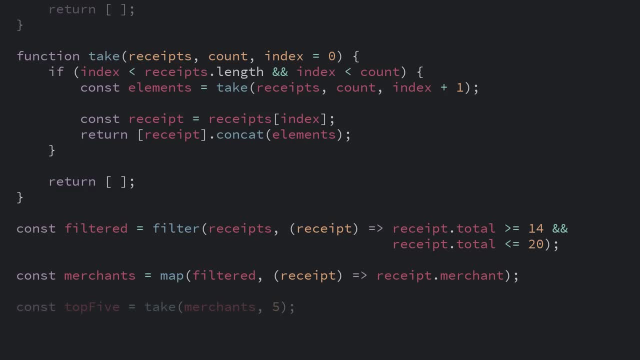 Take would give us up to the count elements from the array. We can chain that on as well. So now you can see that we basically created a data pipeline here Where we have an input state. We filter it down to what we want, Map the types of the values to what we want. 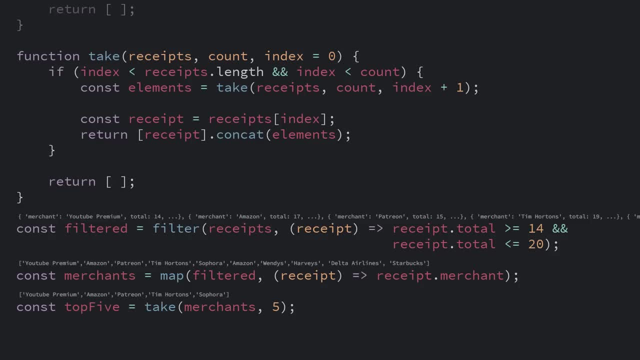 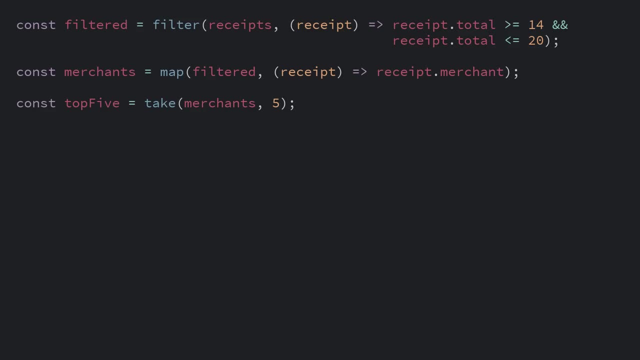 And then take the first 5 to display Our code, clearly declares what we want to happen And all the complexity of how this is done. So what we've done is behind the scenes in our fundamental functions. So we've just derived these functional style fundamentals ourselves. But these are also 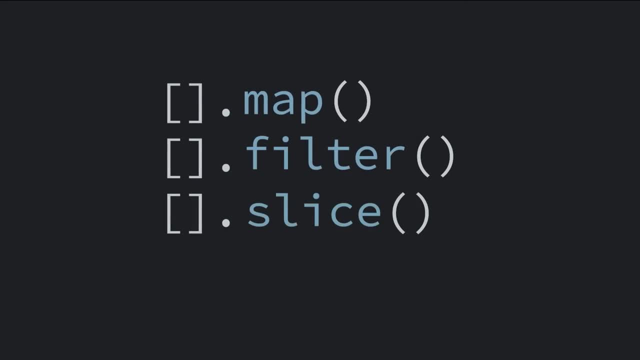 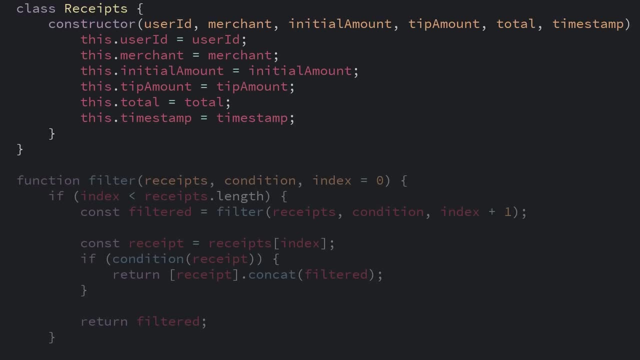 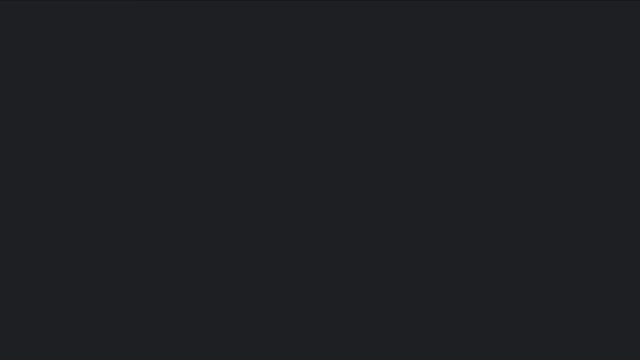 built directly into JavaScript, So let's take a look at how to use those to create data pipelines. But first, what's our goal with these receipts? We have this amazing new startup idea that solves a uniquely American problem in an American way. In the US, when you're in a restaurant, you need to fill a tip menu. 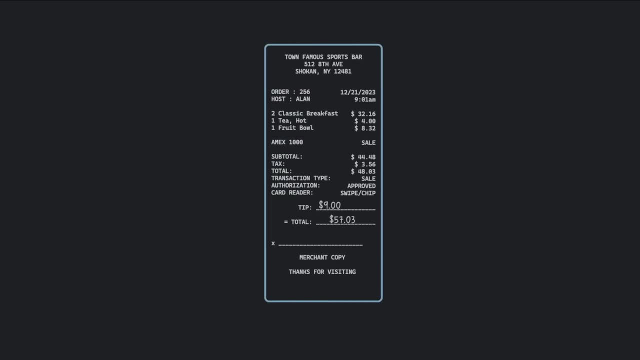 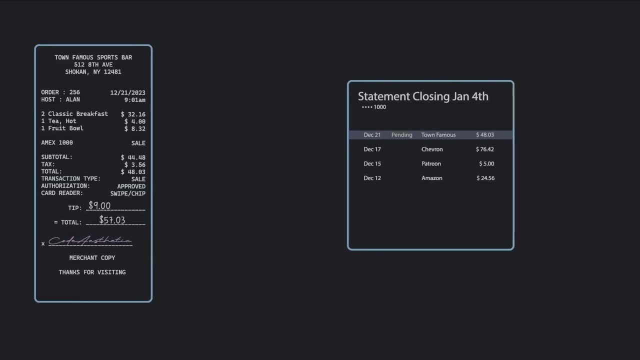 You can do this manually by writing the tip in total. This is effectively a mandatory fee on your meal enforced by social shaming. Your card is initially charged for the total without the tip, But several days later the updated total with your hand scribbled tip will show up. 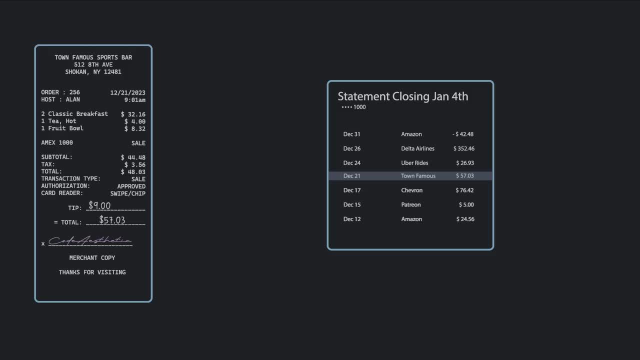 on your credit card. The problem here is that no one is really going to check whether their tip was accurately reported when their transaction was settled. So in theory, a company or disgruntled service staff could simply enter a bigger number, taking more of your money. 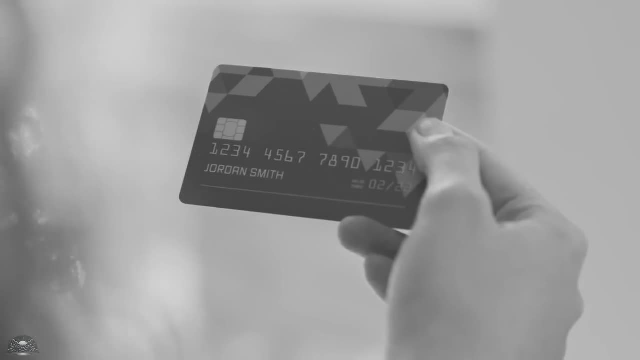 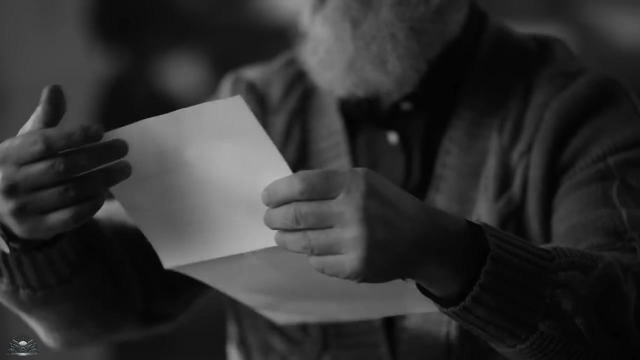 Are you worried about losing your hard-earned money to restaurant credit card fraud? Black Sky Financial finds these small, family-owned mom-and-pop restaurants and sues them for everything they have. The proceeds from the destruction of people's dreams are then equitably distributed to you. 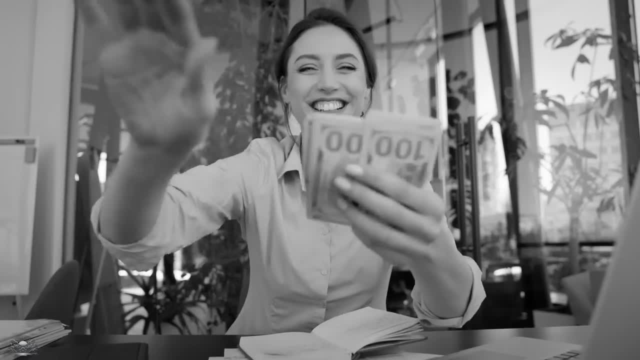 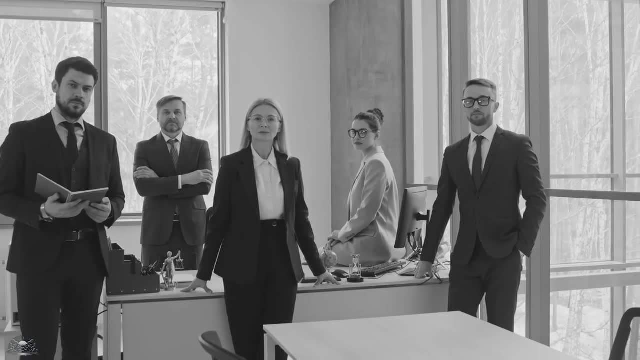 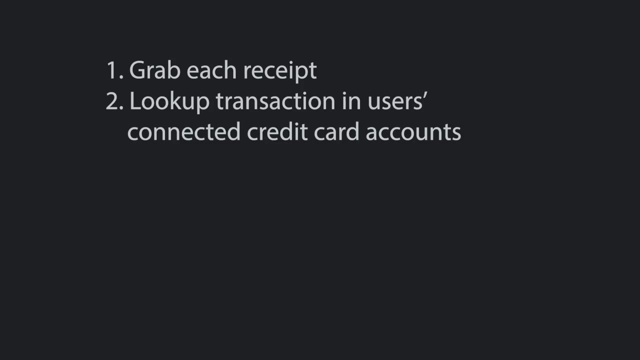 the user of the app based upon how many receipts you've submitted. Sign up today and start submitting receipts, and know that you're helping prevent credit card fraud in your community. one lawsuit at a time. So yeah, to pull this off, we basically need to grab each receipt, look up the transaction. 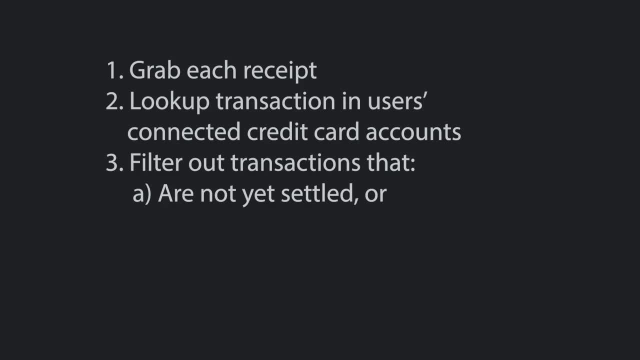 in the user's connected credit card accounts, filter out the transactions that haven't yet settled or whose totals match correctly, sort them by the most egregious discrepancy and then take the top 10.. Then we display them in a dashboard, so our army of lawyers can get to work fighting. 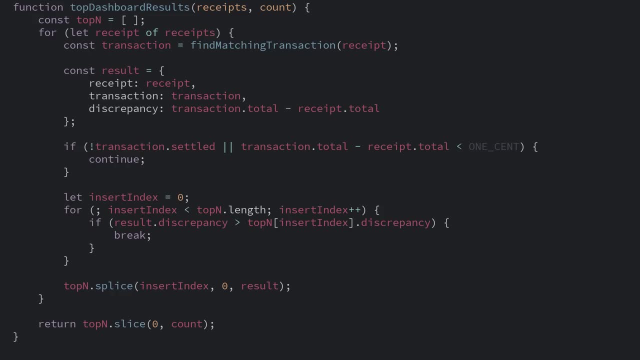 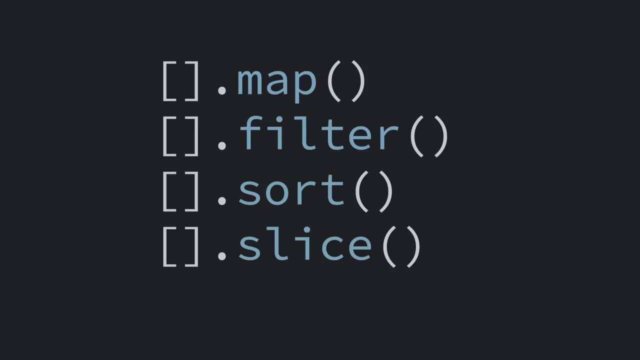 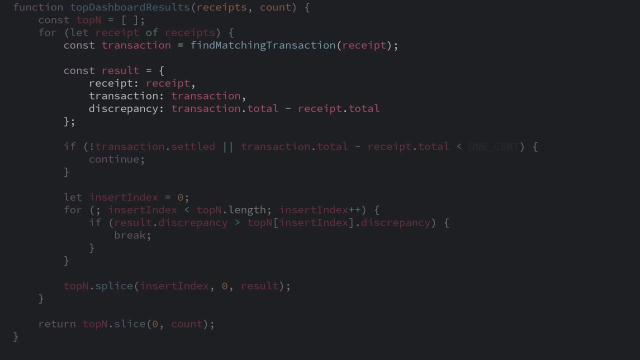 the good fight Here's that code written in a procedural way. Let's change this to the functional approach. In modern JavaScript, all the methods that we need are already built in and are also methods directly on arrays. For each receipt we eventually want this result object that contains all of the relevant. 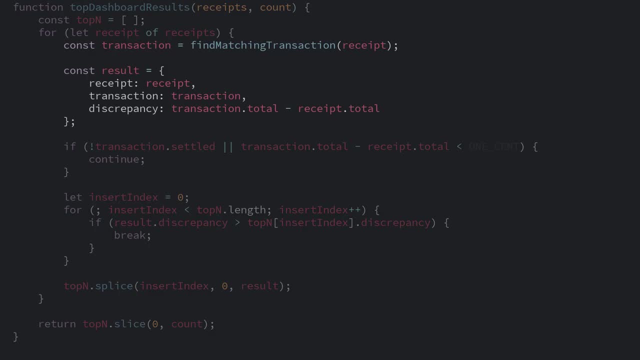 information, The receipt, the final transaction and the discrepancy. So we can just map our receipts to that. We can use the built-in map method on our array to transform the array into our list of objects. The map method takes a lambda function for transforming our receipts into those results. 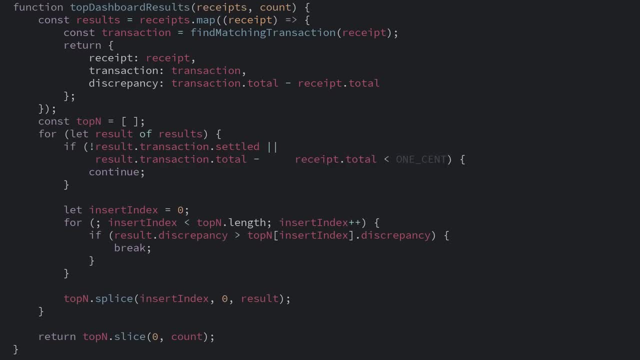 We can also use this method to change the amount of receipts that we want to keep or change the amount of total receipts that we want to keep. This condition is skipping over the transactions that aren't yet settled or don't have a difference between the receipt total and the final total on the transaction. 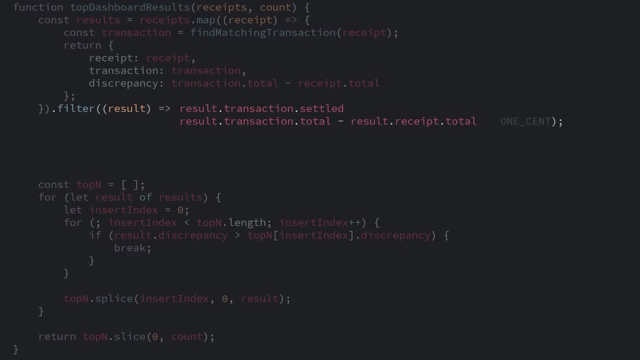 So we can just change this to a filter. We'll need to inverse the condition, since it now describes what to keep instead of what to ignore. This code basically just ensures that the list is sorted from biggest to smallest, So we can replace this with a sort on our filtered list. 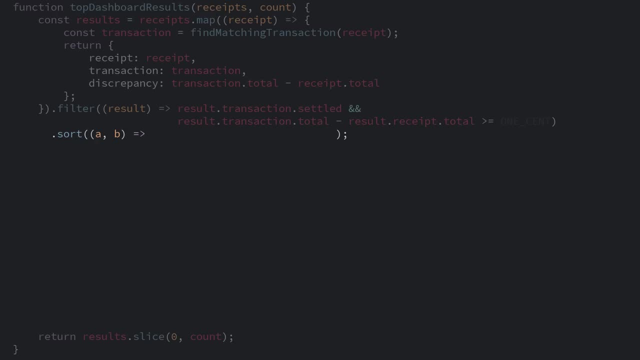 The sort takes a function that tells the sort function how two elements should be ordered. It gives you two items and asks for a negative number if a is less than b and a positive if a is greater than b. You typically get this by subtracting b from a. 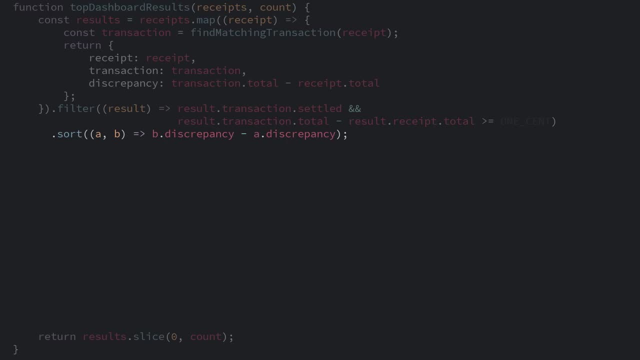 But since we want things ordered big first, we'll flip this and subtract a from b, And then we only want count number of elements, which we can get with the slice method, which we were already doing here. So we'll just add that into our pipeline. 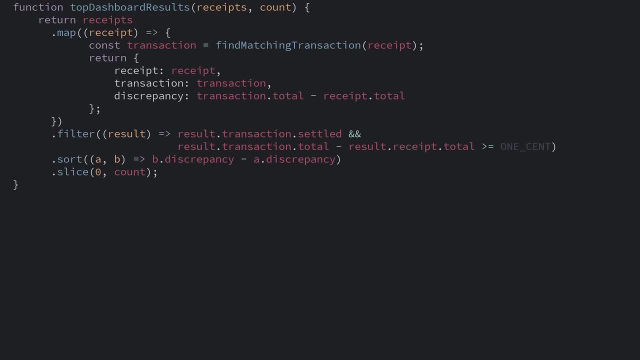 And voila, After we make the formatting a bit more pretty. all of that is written only in 12 lines. Functional programming lets you rewrite things into a beautiful pipeline for your data And, honestly, most of programming jobs are really just taking data from source A doing. 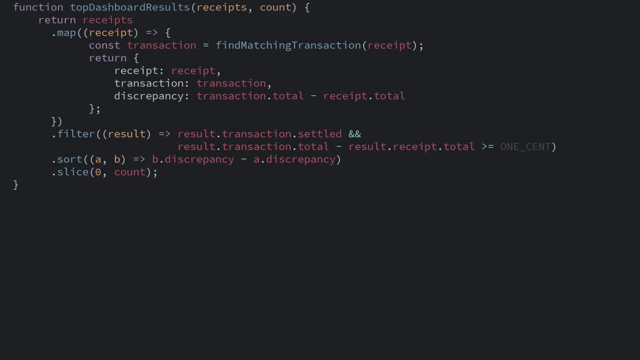 some transformation, filtering and sorting and then putting it in place B A lot of the time, we're just sophisticated plumbers. If you'd like to try out some functional programming like this, I put some experiments on my website or you can follow me on Patreon. 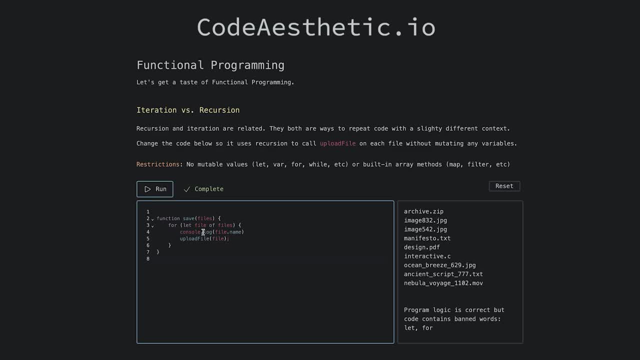 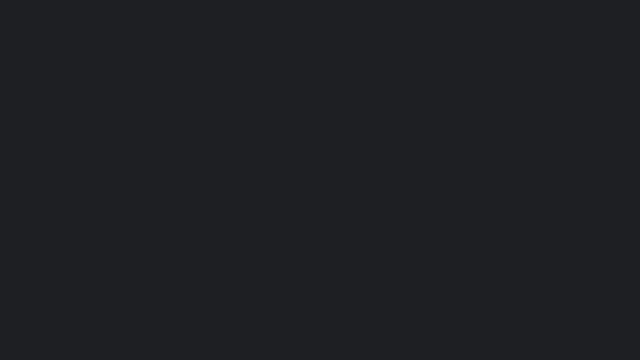 I give you some procedural code and ask you to change it so it doesn't use any for loops or while loops. If you're curious, check them out at codeaestheticio. Dear Functional Bros, Sometimes I feel like you focus on the complexity and mathematical elegance of functional programming. 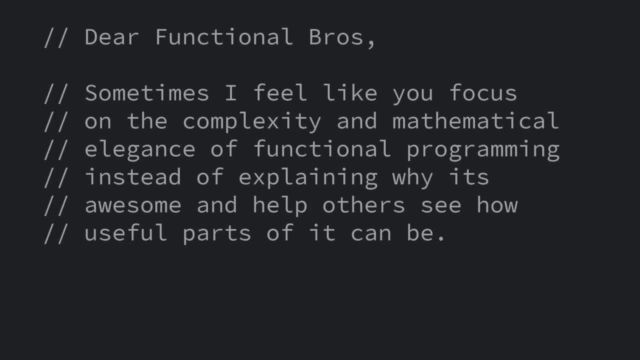 instead of explaining why it's awesome and help others see how useful parts of it can be, Maybe we need a special F-BRO signal to let others know that you're also a secret F-BRO and that you're a real F-BRO. 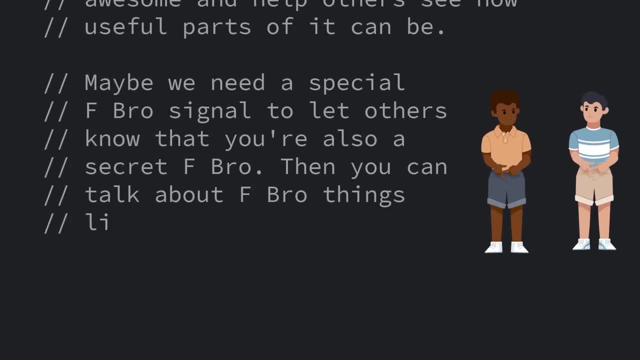 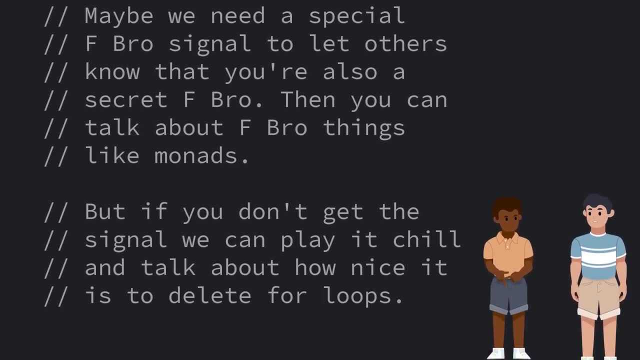 Then you can talk about F-BRO things like monads, But if you don't get the signal, we can play a chill and talk about how nice it is to delete for loops, Pure functional programming, where you cannot mutate any state or have any side effects. 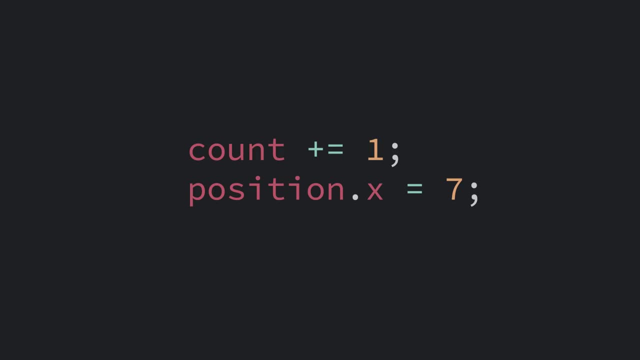 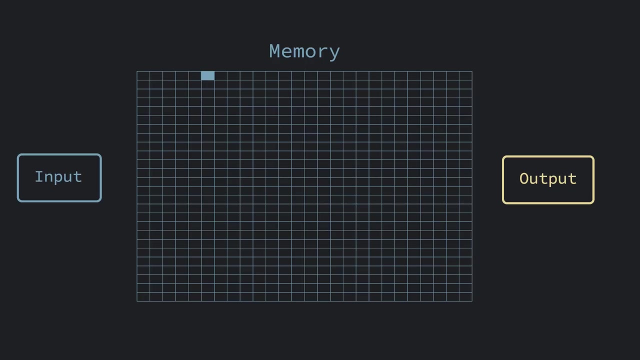 is kinda awful. The issue is it's fake. Computers fundamentally have state. I mean literally the whole von Neumann architecture is where you have one giant state in memory and then little instructions. Input is non-deterministic and any output is forcing some side effect. 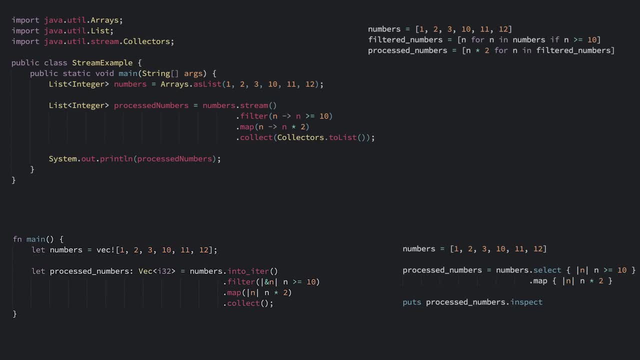 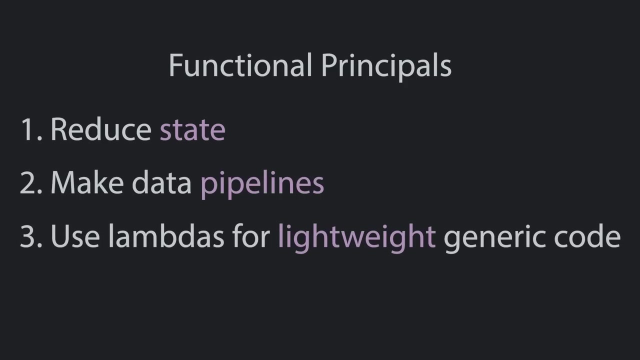 Pure functional programming is still mostly academic, But what has been happening is the best parts of functional programming have been extracted and injected into our most popular languages. Like always, balance is key, and adopting some of the principles like reducing state and formulating data pipelines in your programs where it makes sense can bring huge benefit.